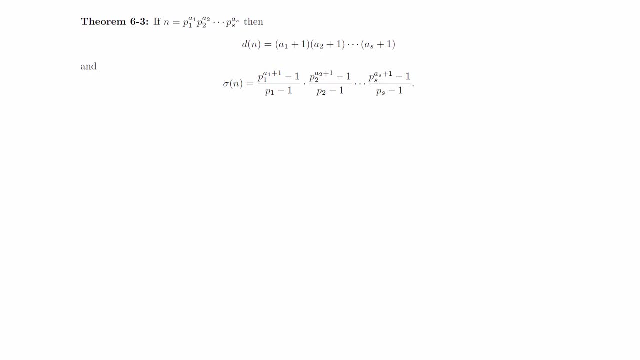 and sigma of n, given that we know its prime factorization. Let's start with this statement by induction on the number of distinct prime factors of k. When k is equal to 1, we have the cases that we have just discussed. So now suppose that the theorem is true when there are k or fewer distinct prime factors. 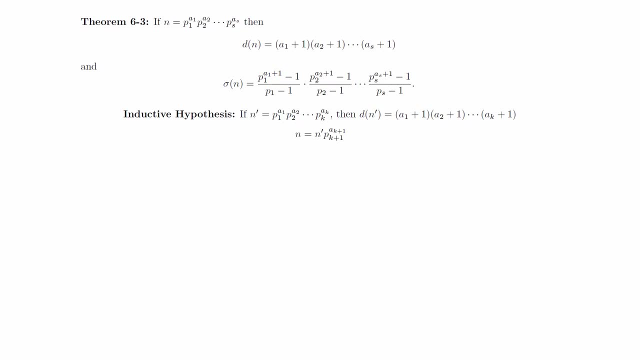 and suppose that n equals n prime times p sub k plus 1 to the a sub k plus 1, where n prime has k distinct prime factors and p sub k plus 1 does not divide n prime. We need to use this notation in order to be consistent with the notation provided in the 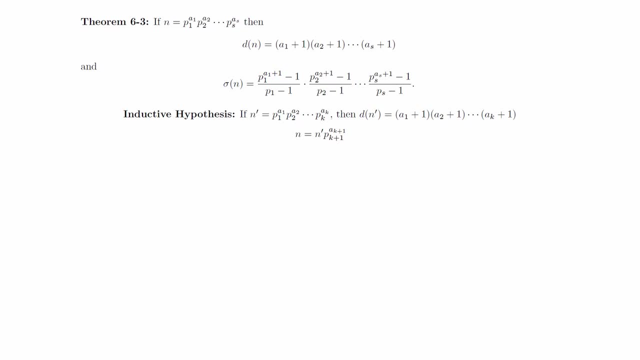 statement of the theorem. We want to figure out what the prime divisors of this number n are. Suppose that d1, d2, up to dt are the divisors of n prime and consider this chart of values. The divisors of n prime are written across the top of the chart and the divisors of p, sub k plus 1. 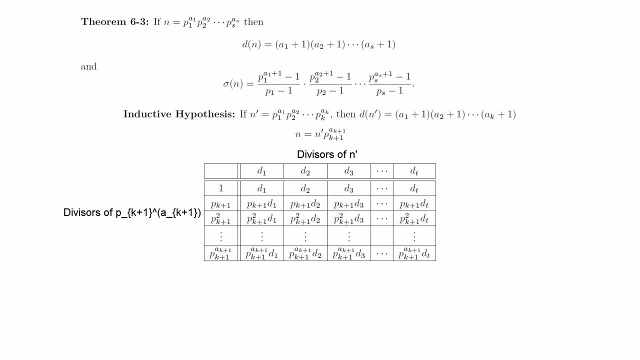 to the a sub k plus 1 are written down. the left column. Every divisor of n is listed exactly once in this chart. We can see this since every divisor of n will have some power of p sub k plus 1 in it where that power might be zero. 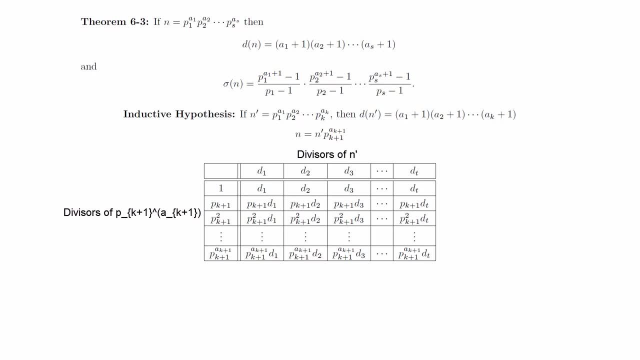 The divisor we are left with after factoring out the powers of p sub k plus 1 will be some divisor of n prime. As an explicit example, here's how the chart looks for: n equals 90, where n prime equals 10, p equals 3, and a is equal to 2.. If we pick an arbitrary divisor of 90, such as 15,. 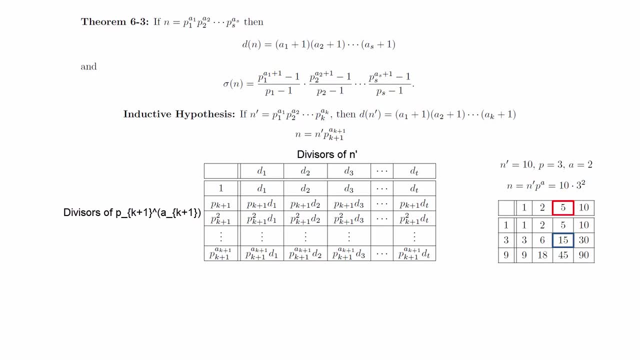 we could break that number into a product of two terms, one of which divides n, prime or 10, and the other of which is a power of p or 3.. Once we do that, we can see that this term appears in. 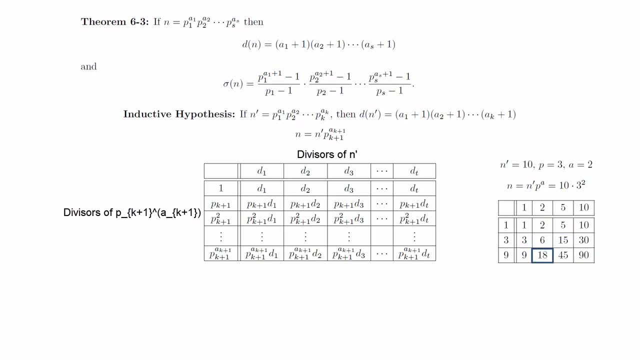 the chart in the corresponding position. We can also go in the other direction and pick an arbitrary value in the chart and see that it comes from the product of two terms, one of which divides n prime and the other of which is a power of p. Now that we know this, we can see that there are d of n prime times a sub k plus 1 plus 1. 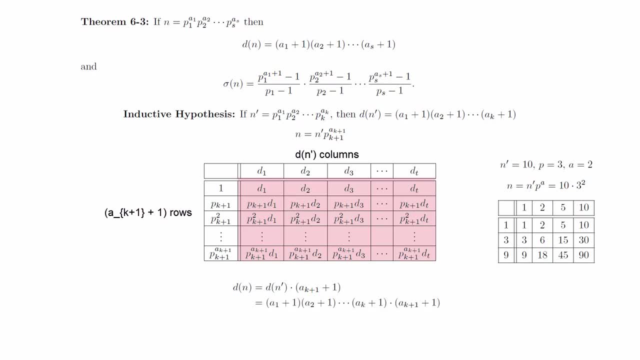 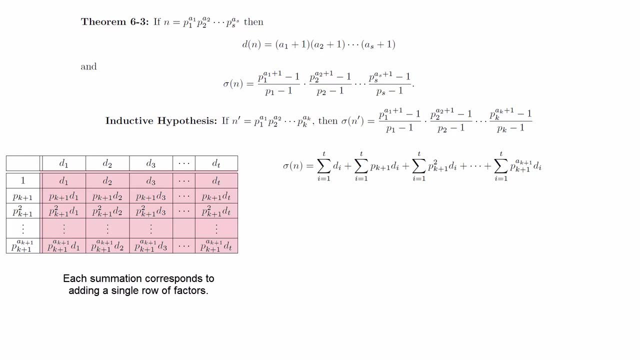 divisors of n, and we can now use the inductive hypothesis to get the desired result. Similarly, we can add up all the values in the chart to compute sigma of n. Although this initially looks messy, notice that by factoring out the individual,